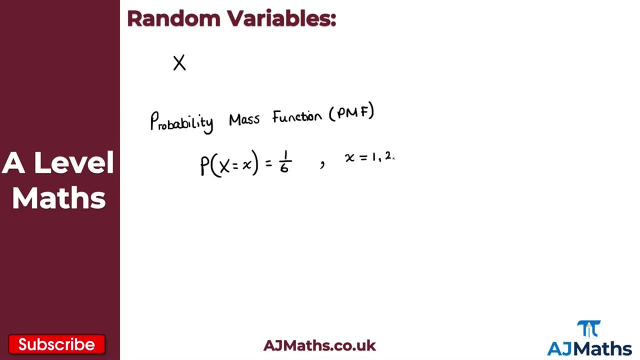 be little x, equal to 1,, 2,, 3,, 4,, 5 and 6.. So those are the particular values that we can get here For our random variables. variable X: okay, now we can also present this in a table. so if we present this in: 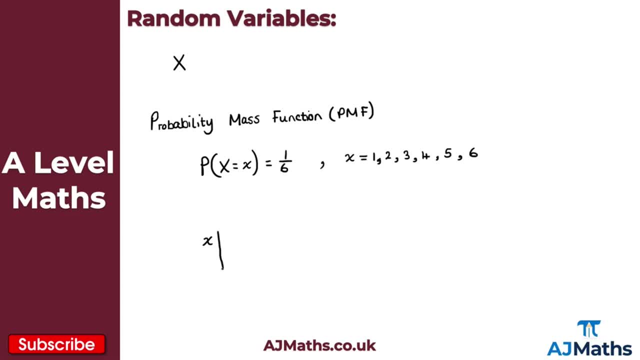 a table here we'd have the particular values that we can take and then the respective probability here for our random variable. okay, so obviously the particular values that I can take are these six values here: one, two, three, four, five and six. what I would recommend is using a ruler, don't do it. 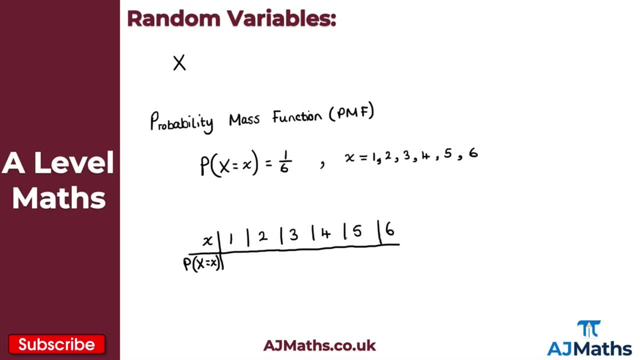 freehand like I'm doing here, I'll make yours look a little bit neater than mine. okay then, obviously, for these respective particular values here, then the respective probability will always be one over six. okay, so, one over six, one over six, one over six. again, one more or two more times, and finally, the last time there. 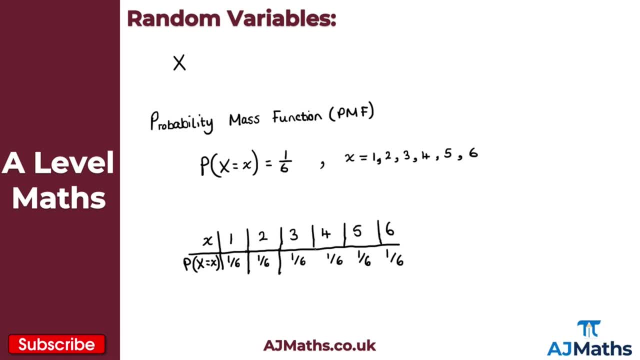 okay. so, if I just close my table off here, we have something that looks like that: okay, so what can we know is here? well, for a random variable, in this case for our random variable X. what you should hopefully notice them is: the sum of the probabilities here will add to one. okay, that might sound obvious, but it is a key fact here: the sum of 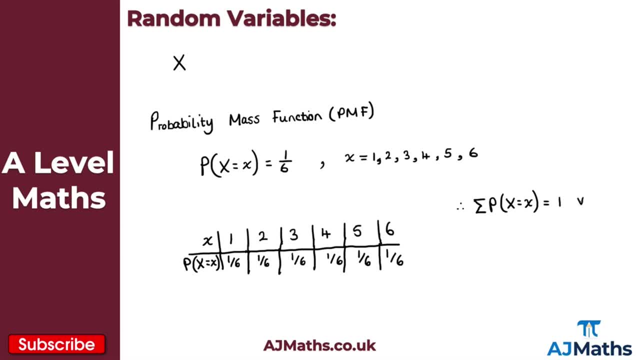 the probabilities here is equal to one for all particular values of x. okay, that is important. and here i just finally give the definition, then, of our probability distribution. we say that the probability distribution fully describes the probability of any outcome in a sample space. okay, so what we've got here, this here what we call our probability. 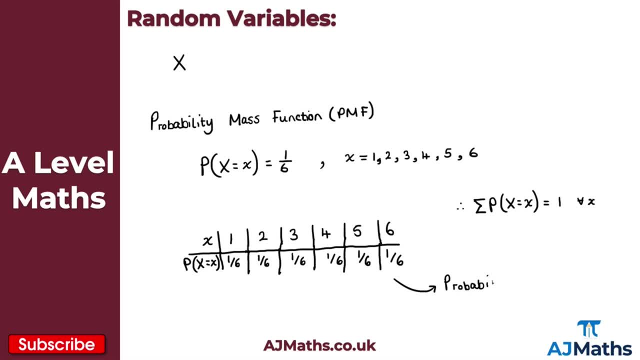 distribution. okay, so let's write this out in full, like we said. that's our probability distribution there. okay, and just one more thing here before we finish. then this here is a special type of discrete random variable. this is a uniform discrete random variable. this is uniform because each outcome here 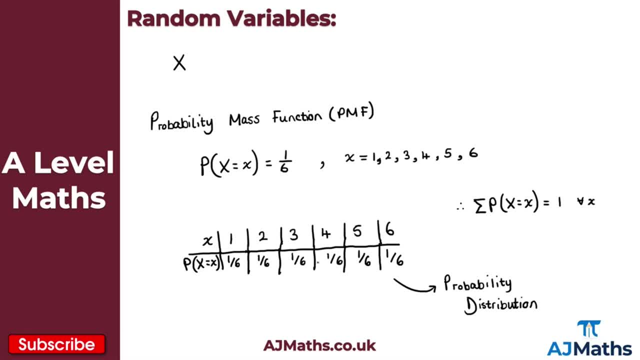 each outcome. here is a uniform, discrete random variable. each probability is equally likely. okay, so if the probabilities are equal like this, that would be a uniform random variable. okay, so that's everything we need there for our introduction to probability distributions. what we're going to do now is take a look. 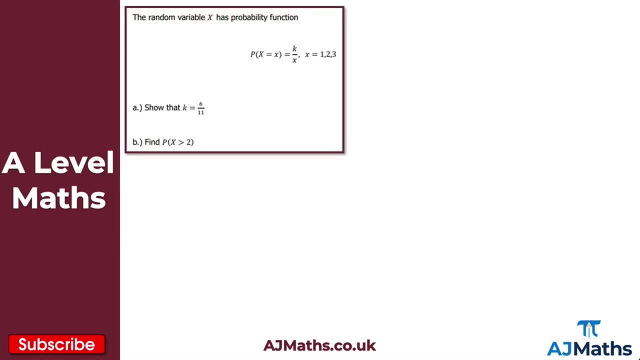 at some practice questions. so if we begin with question one here, then we've got the random variable x, which has probability function given, as we can see here. so for pi a we're asked to show that k is equal to 6 over 11. so to begin with here what we should do is find the 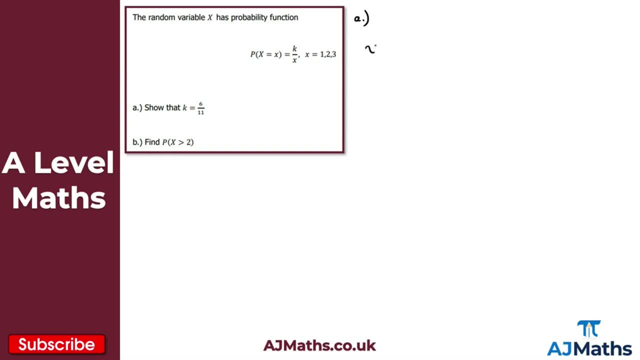 probability distribution in the form of a table. we've got x here and then the probabilities for a random variable here taking these values of x. so obviously the three values we can take here for little x are one, two and three. for one, two and three. so what i would recommend doing like 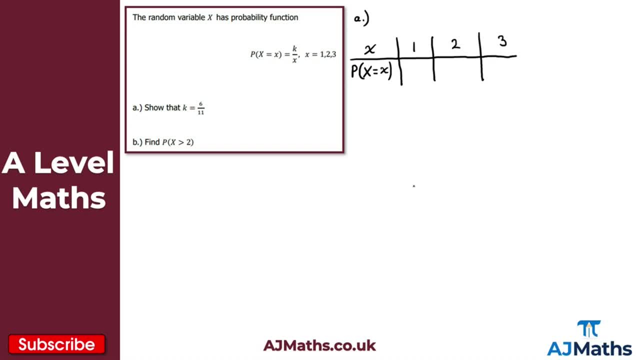 i said before is: do just use a ruler to make it look a little bit neater than i am. when x is one, here we get k over one, which is equal to k. when x is two, we get k over two there, so a half k or k over two, and then finally, finally, here, when x is three, we get k over three or a. 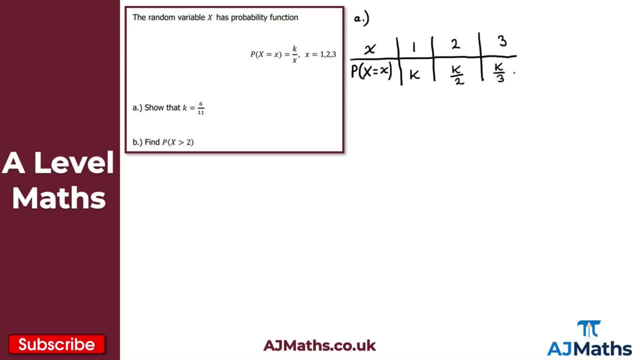 third, k. okay, so what we know here. so some of these probabilities should be equal to one. so the sum of these probabilities here will be equal. one, okay, plus k over two. plus k over three is equal to one. we write that down here: k plus k over two. 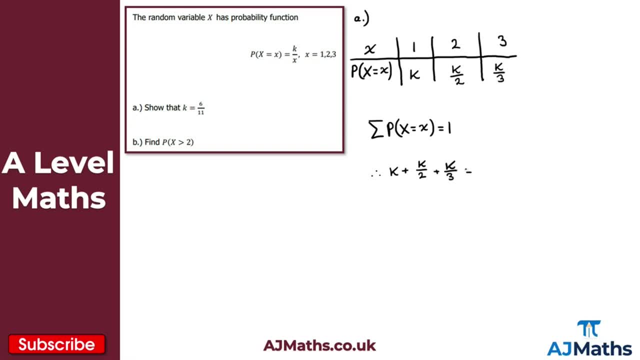 plus k over three, and that's equal to one. okay, what you can do here is factor the k out. i'm gonna get k lots of. one plus a half plus a third, and that's equal to one here. but one plus a half plus one over three, that would give me eleven over six. 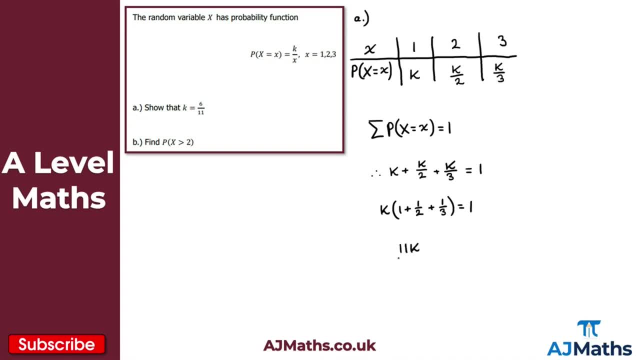 what i'm gonna get here is 11k over six is equal to one. so i want to solve for k here. i just need to divide by eleven over six, or just times three by six first, then divided by eleven. either way, you'll get the same thing here and you'll get that k is equal to six over eleven. 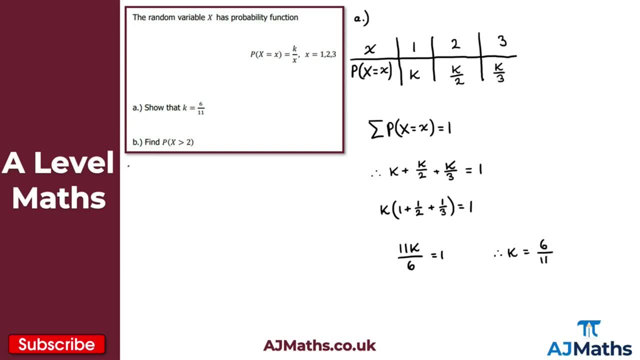 okay, so that's part a done there. that's our solution, hopefully nice and straightforward. so for part b, then we have to find the probability here of our random variable x being strictly greater than 2. let me just write this down here. so the probability of our random variable x being strictly greater than 2. 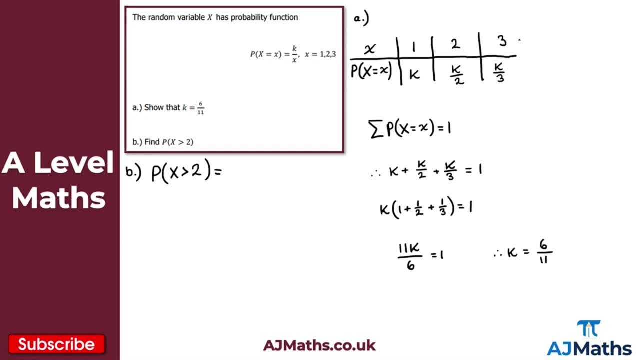 well, that means the only possible option we have here is when x is equal to 3. okay, that's equal to the probability of our random variable x being equal to 3, which is k over 3. but we know that k is equal to 6 over 11. that's going to be 6 over 11 divided by 3. that's going to give me 6 over 33. 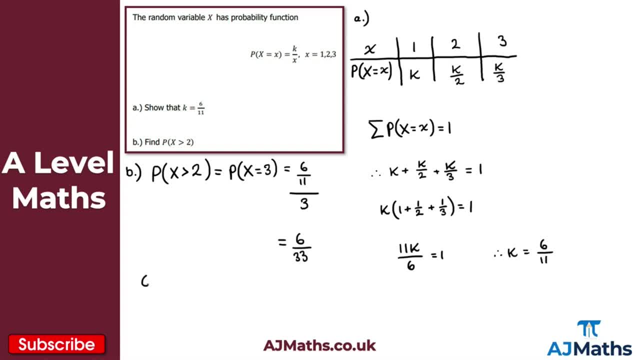 there okay, because that's the same as 6 over 11 times 1 over 3, which would give us the 6 over 33 there. okay, and there we have it. so that's our solution to c and that gives us the solution there to question 1. 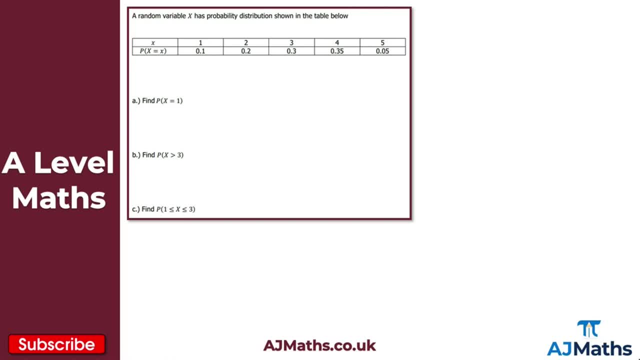 and finally, if we take a look at the very last question, here we've got a random variable, x, which has probability distribution shown in this table below. so we've got three parts to this part a: we have to find the probability that x is equal to 1. so for this question, hopefully nice- 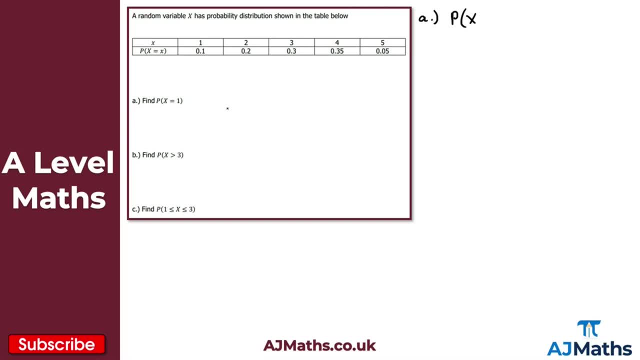 and straightforward. we are just using this table here to answer a, b and c. so the probability that our random variable x here is equal to 1. well, that would just be this case here. okay, so in that case our probability here will simply be 0.1. that's our solution to a for b. then the probability of x here or our random 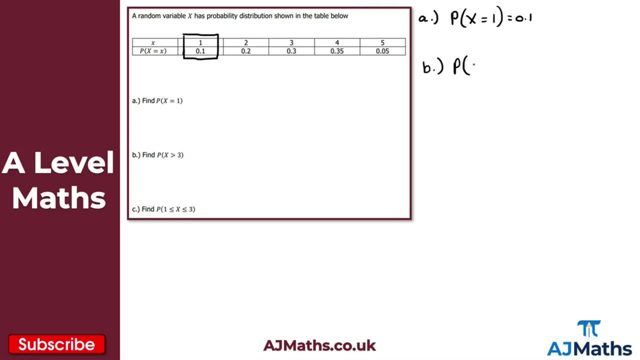 variable x being strictly greater than 3, the probability that x is truly greater than 3. we've got two options here. we've got this one here- our probability of 0.35, and this one here- our probability of 0.05. so what we need to do here is just add those together.